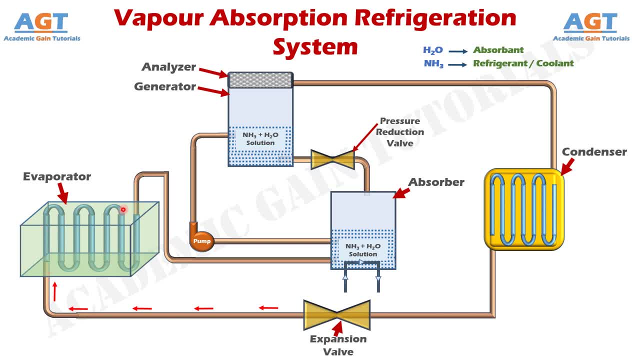 We all know that the main cooling effect or refrigeration effect always occurs in the evaporator. So when this low pressure, very cold, chilled, low temperature liquid ammonia will enter the evaporator coils, it will absorb all the heat present in the surface of the evaporator coils. 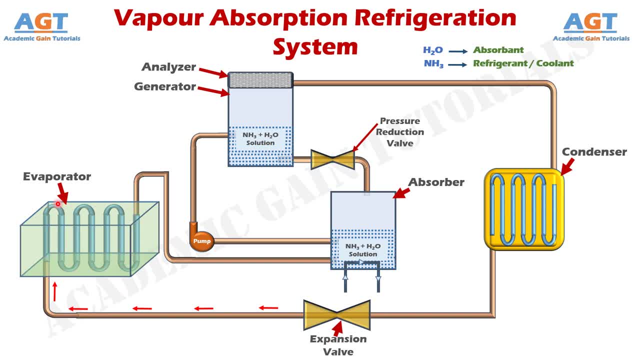 By absorbing all the heat from the surrounding region of the evaporator. it will absorb all the heat present in the surface of the evaporator coils, the evaporator coils. this cold, chilled liquid ammonia will turn into low pressure ammonia vapor inside these coils and the surrounding surface of the 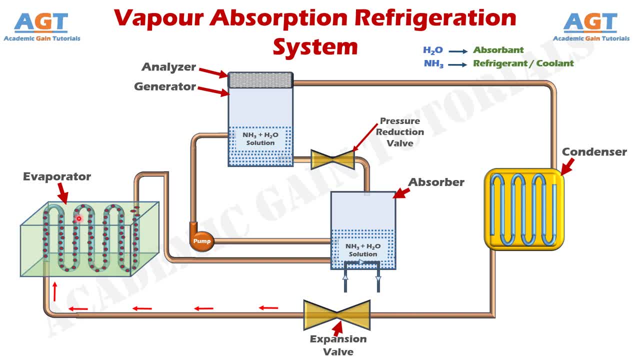 evaporator will become cold by losing the heat to this liquid. thus the cooling effect, or refrigeration effect, has occurred in the evaporator. after that, this low pressure ammonia vapor will leave the evaporator and enter the absorber through this connecting pipe. the absorber already has a weak solution. 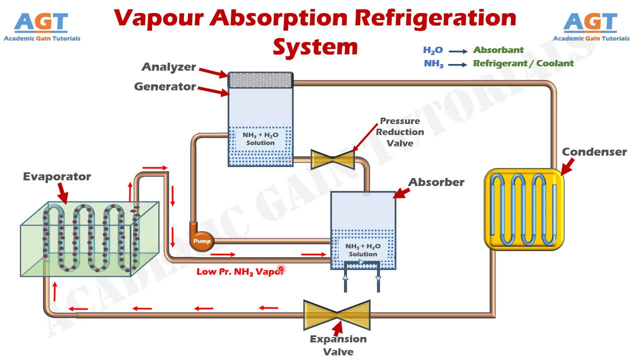 of ammonia and water inside it, and when the slow pressure ammonia vapor enters the absorber, the water present in the weak solution of this absorber will start absorbing this ammonia vapor and the weak solution will gradually convert into a strong ammonia water solution. the more ammonia vapor coming from the 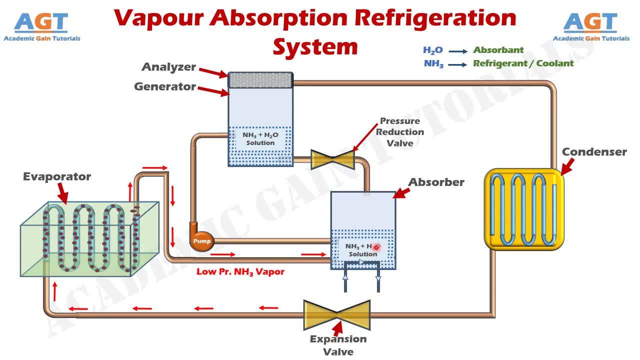 evaporator is absorbed by water from this weak solution, the stronger this solution will become. but when water absorbs ammonia vapor, it also liberates heat. that is when water will the incoming air that is now世을 Act. you could turn down from this water vapor, so we will. lovers campaigning per. 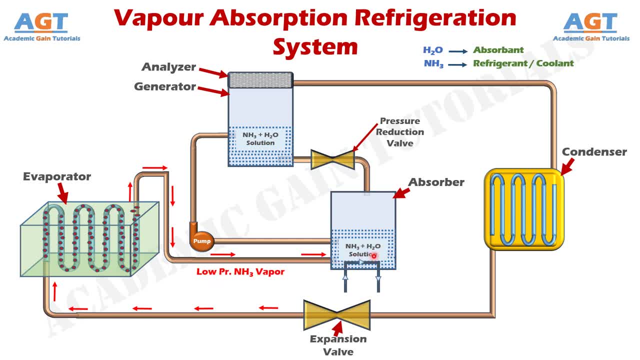 water vapor, it will also liberates heat. that is when water will absorb the incoming water liquid theld Architecture of warm water so it will turn warmness. when this water vapor will not change and when water will absorb ammonia vapor, it will lose temperature. ammonia vapor, it will produce heat which will increase the temperature of the 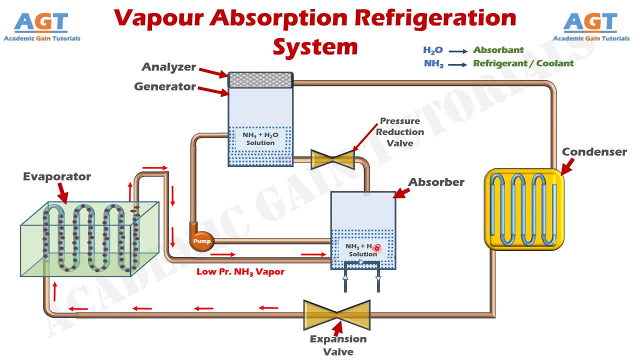 solution. and when the solution becomes hot, gradually the capacity of water to absorb ammonia decreases. so to keep the temperature of the solution to an optimal level, a supply of cool water is provided through this pipe, so that this external supply of cool water through this pipe carries away heat from the 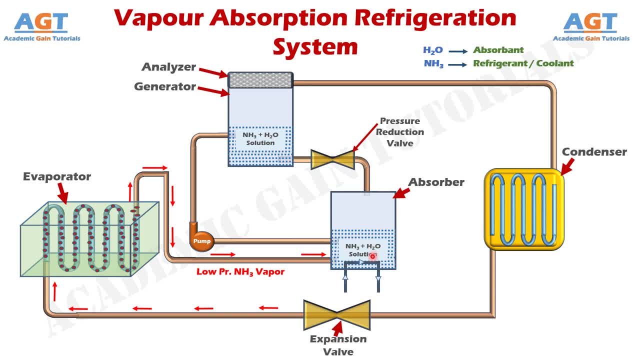 solution and thus water regains the capacity to continuously absorb incoming ammonia vapor. beside this absorber there is a pump. now, when power is provided, then this pump starts working. then, using this pump, this strong solution of ammonia and water will be pumped from this absorber to this. 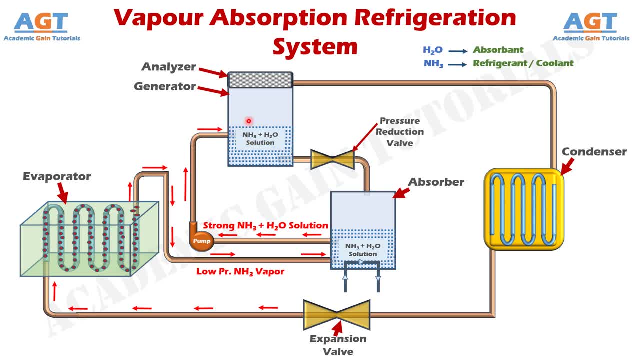 generator. so the function of this pump is to transfer the solution from the absorber to the generator. we provide auxiliary heat or external heat to this generator, either by using steam or hot water or any heater- gas burner, air heater explained below, etc. So when the solution of ammonia and water reaches the generator and heat is applied, 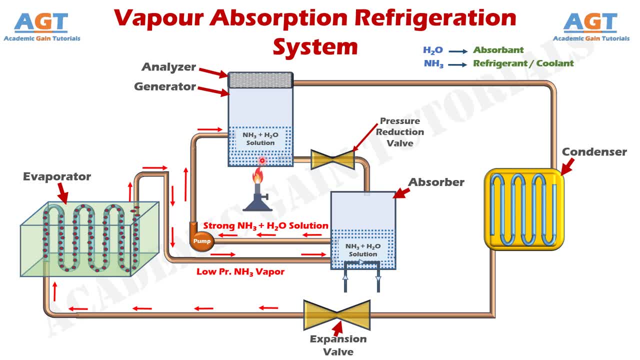 to this solution from the external source. both ammonia and water from this ammonia water solution turns into vapor inside this generator. Actually, ammonia turns into vapor faster than water and water takes comparatively more time to completely turn into vapor, but eventually both ammonia and water will turn into vapor when heat is provided. 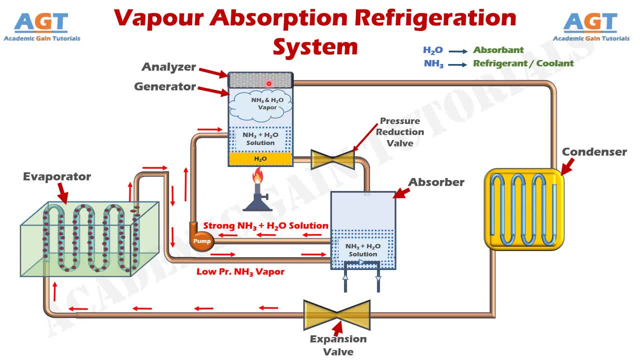 Now here we also have an analyzer on the top of this generator. When this vapor of ammonia and water tries to pass through this analyzer, only ammonia is allowed to pass through. the analyzer continuously condenses the water vapor and sends water back to the 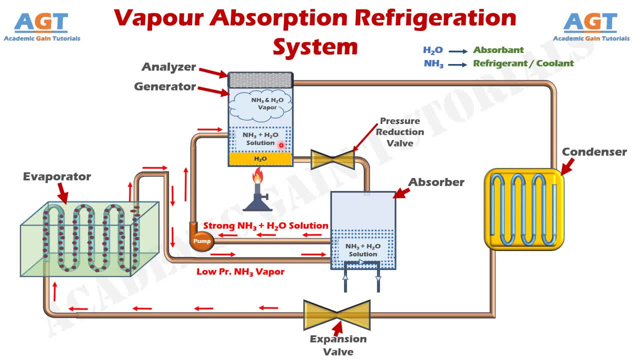 generator. This is because if water vapor enters the system, it can decrease the efficiency of the refrigeration system. or if larger quantity of water vapor enters the system, then the system could be damaged. Thus the analyzer separates water particles from ammonia vapor and only lets ammonia to pass. 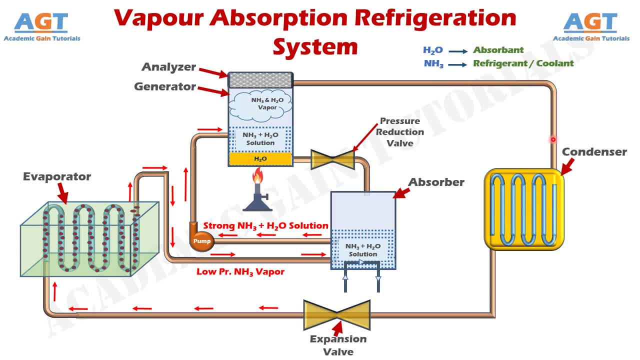 through to the next components through this pipe for further process and the analyzer sends water particles back to the generator. Then from this generator the residue weak solution of water and ammonia accumulated here will be passed back to the absorber, again passing through this pressure reducing valve. So here the high pressure, high temperature. 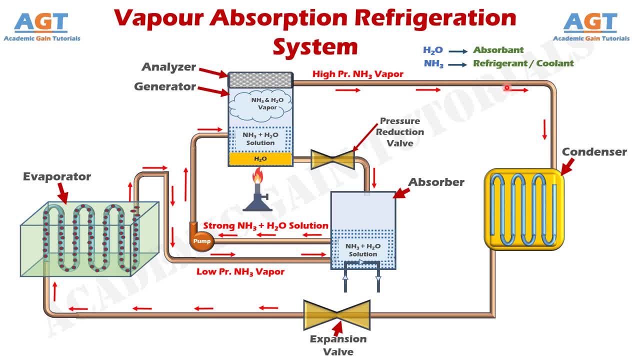 pure ammonia vapor coming out of the generator will now enter into this condenser. Here we have a condenser. When high temperature, high pressure ammonia vapor enters this cold condenser, then the condenser absorbs the heat from the ammonia vapor and completely. 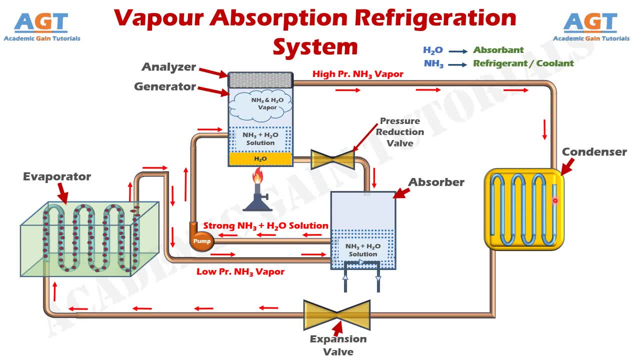